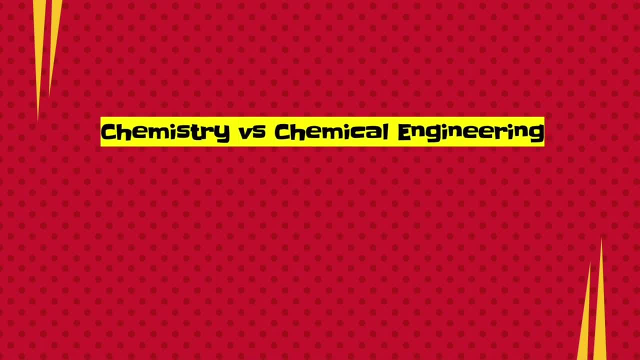 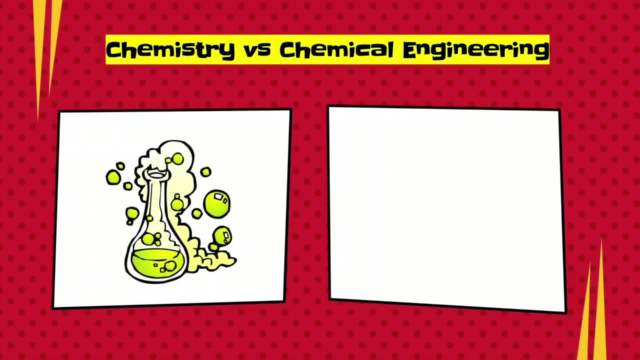 engineering are two very different things. Chemistry is the study of reactions and the discovery of reactions. Well, chemical engineering is taking the reactions that chemists have came up with and trying to optimize them, then put them in a calculated position where you can rely on them. 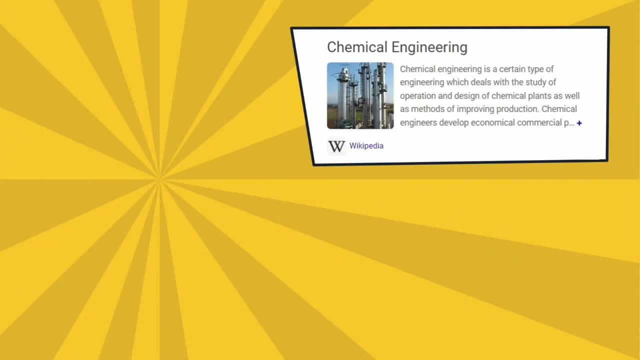 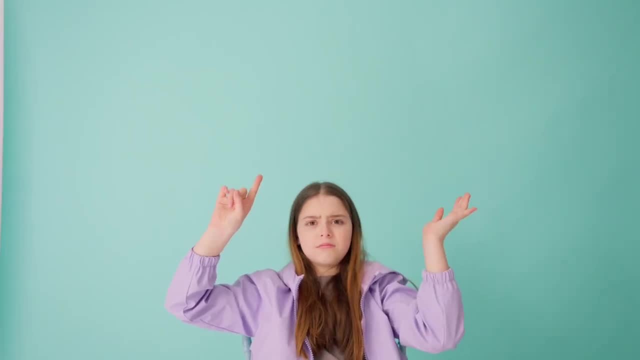 If you search online, Google might show you this, this, this and this, But we are pretty sure that you are still having confusion about what is chemical engineering. No worries, let us answer your questions. Thank you for watching. See you in the next video. Bye. 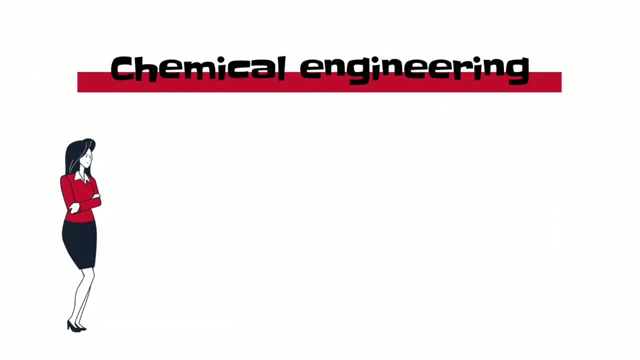 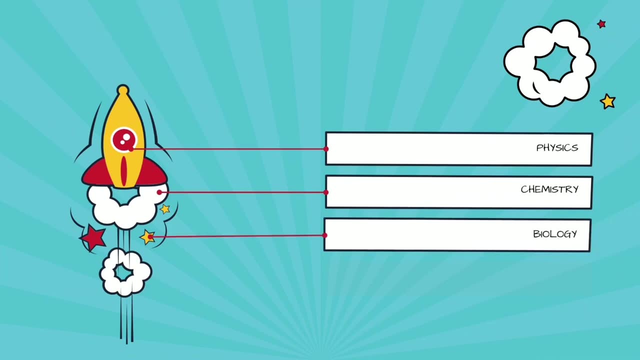 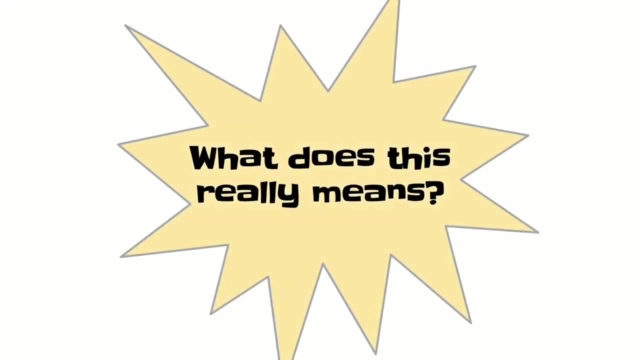 What is chemical engineering? Chemical engineering creatively combines the three basic physical sciences- physics, chemistry and biology- along with mathematics, to address the world's need by creating new technology and improving existing technology. But what does this really mean? It is providing clean water and sanitation to communities. 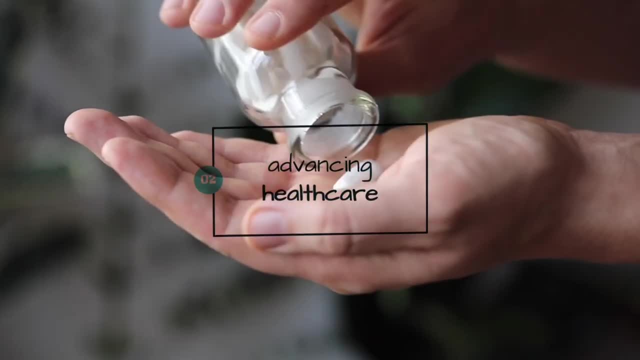 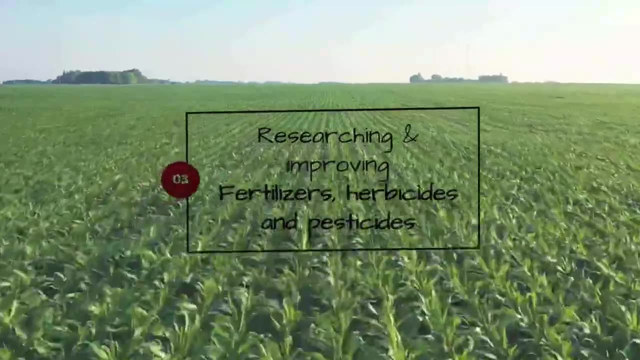 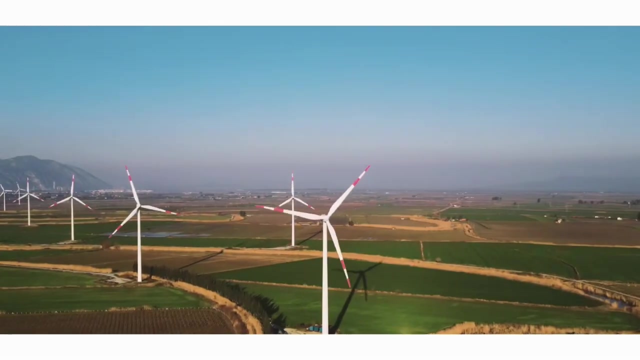 It is advancing healthcare by developing drugs to cure diseases. It is researching and improving fertilizers, herbicides and pesticides to make crops hardier and more disease-resistant. It is designing greener products and processes to control pollution And finding new ways to generate energy. Basically, chemical engineers are improving. 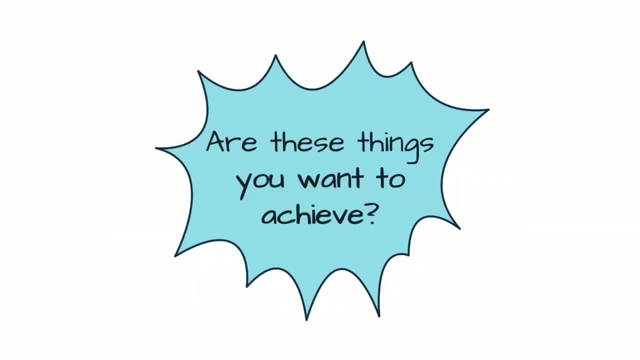 the quality of life in the environment we live in. So these things you want to achieve. You might become a chemical engineer, if you like, Combining maths and science, designing efficient processes, having a curious mind, developing your ideas into usable products, taking your ideas out of the glass and into 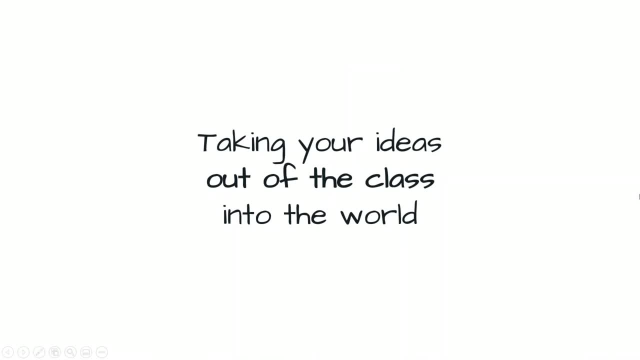 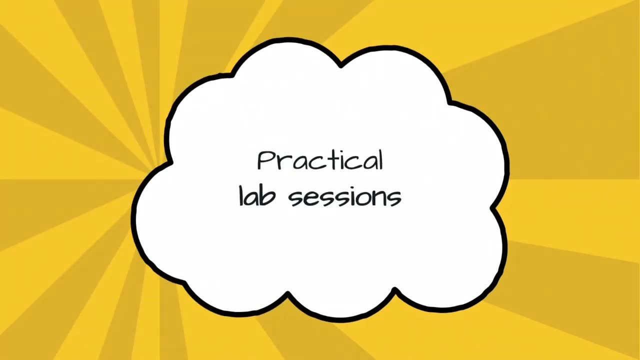 the world with real-life applications. studying chemical engineering in books. learning theory in lectures. applying what you learn in practical lab sessions. solving issues in problem classes with your peers. exploring new technologies. developing industrial strategies. understanding concept to design processes and products. working in teams to solve. 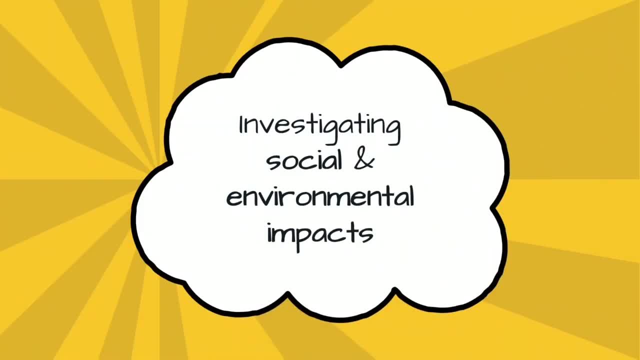 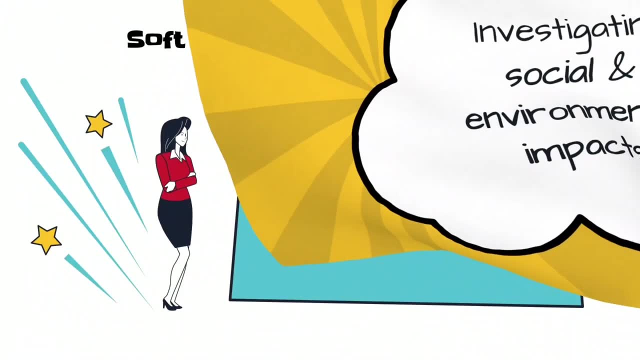 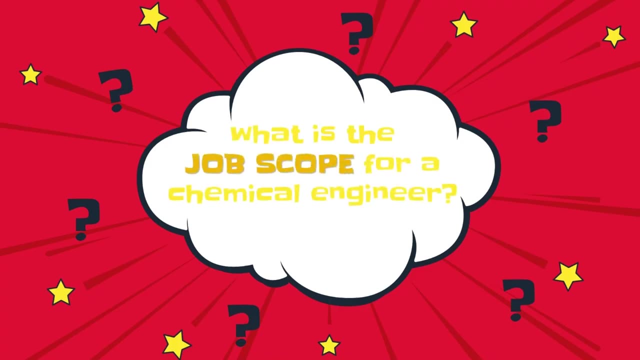 engineering challenges and developing new technologies- This is what chemical engineering is about- And investigating the social and environment impacts of engineering. By doing these things, you'll gain more than chemical engineering theory. You will have skills in critical thinking, problem solving and project management. Do you know what is the job score? 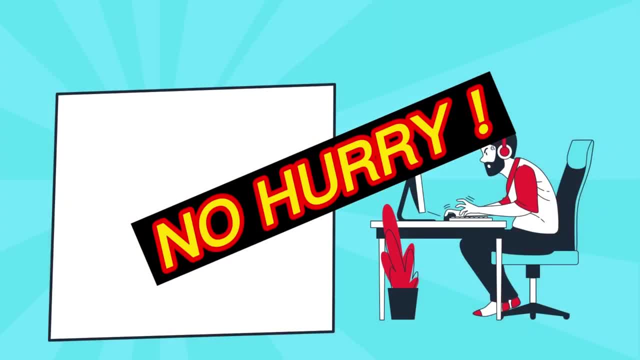 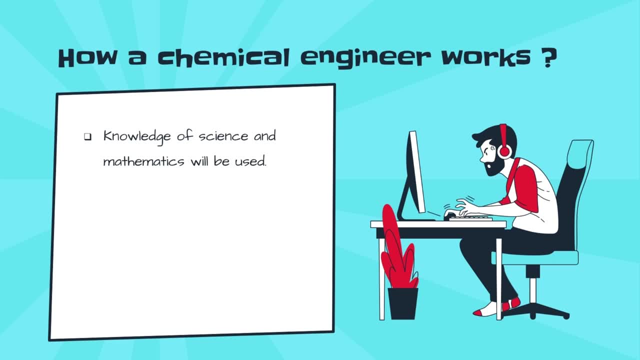 for a chemical engineer. Don't hurry. Before this I will tell you about how a chemical engineer doing a job. In fact, the knowledge of science and mathematics will be used to improve process and equipment used in processing chemicals and find solutions to the problems which make. 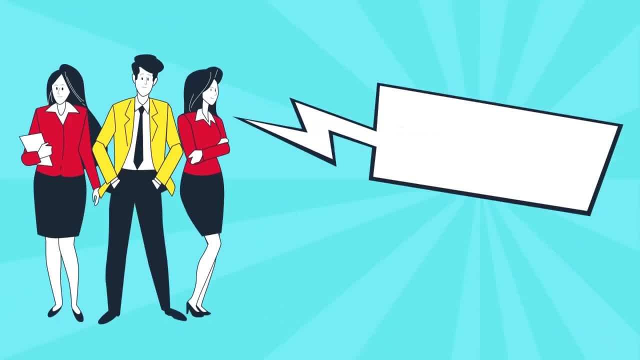 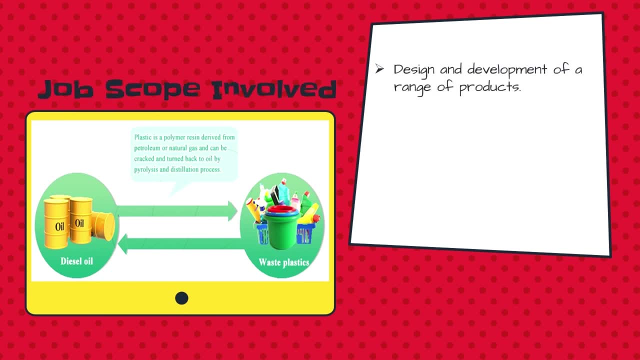 industries face. Now let's move to the part of job scope for a chemical engineer. As a chemical engineer, you will be involved in the design and the development of a range of products. Your work will focus on changing the chemical, biochemical and physical state of a substance to turn it into. 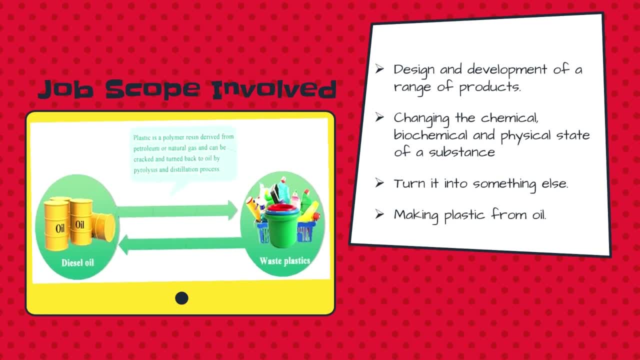 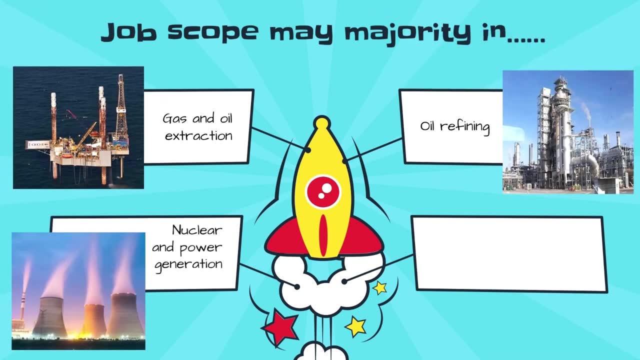 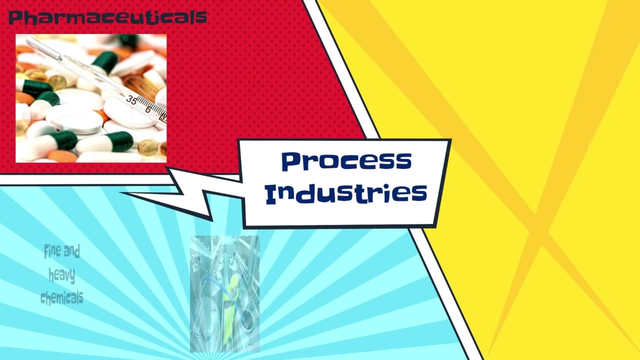 something else, such as making plastic from oil. Therefore, your job scope may majority in gas and oil extraction, oil refining, nuclear and power generation and process industries, which may include pharmaceuticals, fine and heavy chemicals, and also agrochemicals, Other manufacturing. 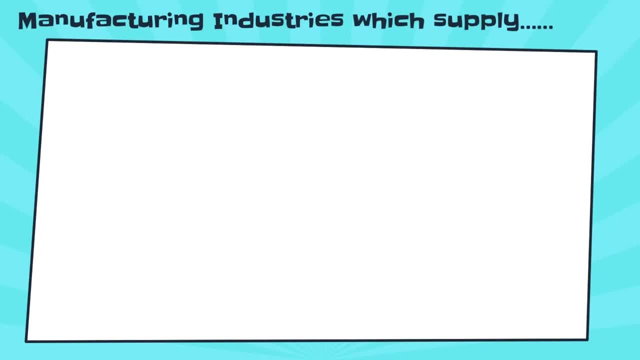 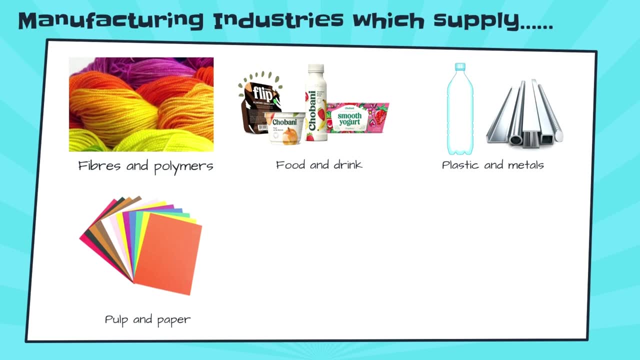 industries that need chemical engineer include those supplying fibres and polymers, food and drinks, etc. You may also be involved in the manufacturing and manufacturing of chemical drink, plastic and metals, pulp and paper, toiletries and water treatment. There are also 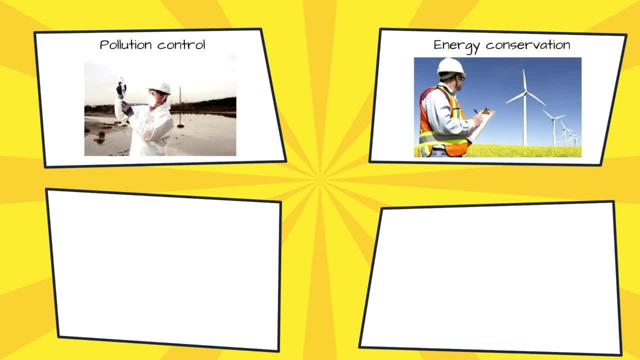 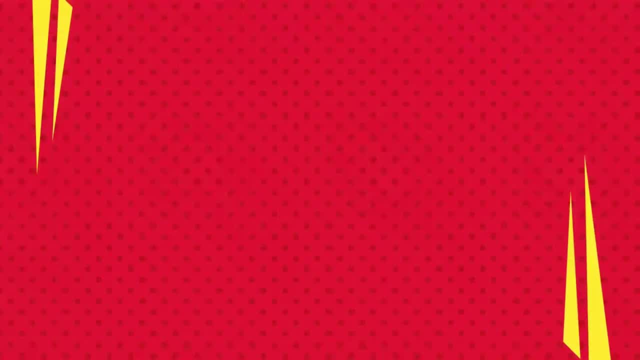 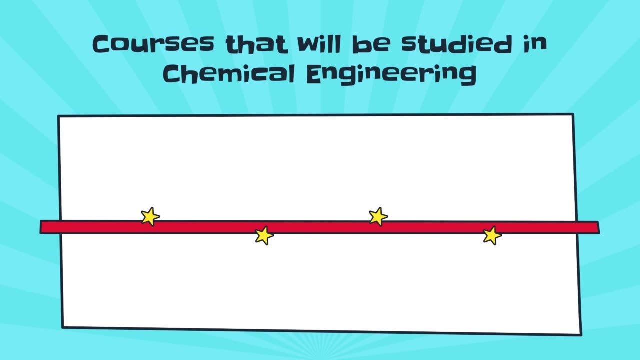 opportunities to work in pollution control, energy conservation, waste recovery and recycling, medical science and so on. Next, I will share some information about the courses that will be studied. in chemical engineering, For example, we will take engineering math, mass balance, energy balance. 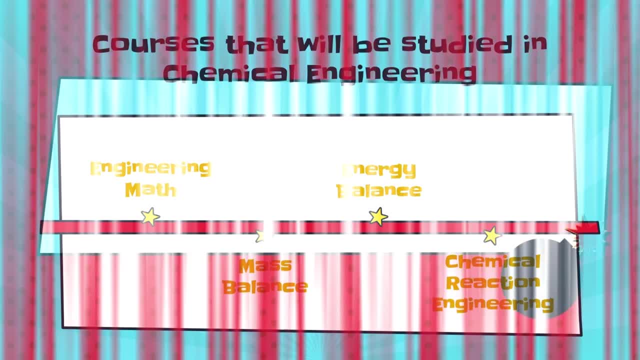 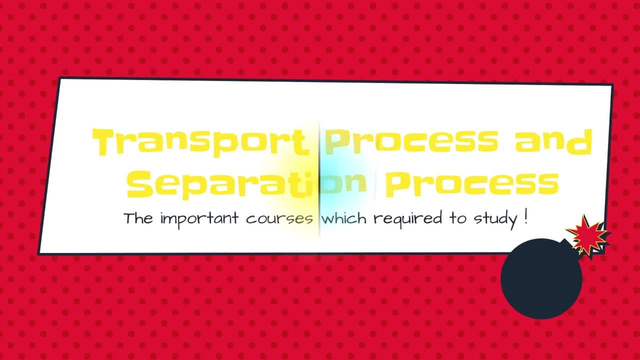 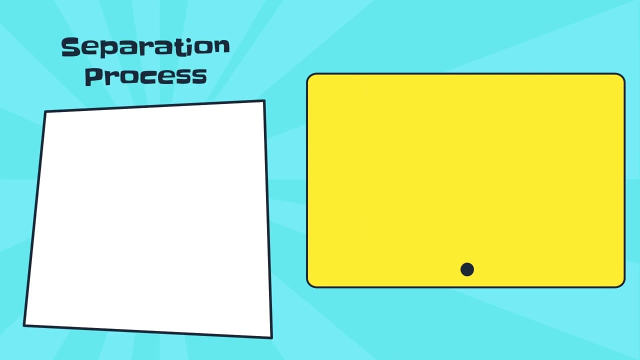 chemical reaction engineering and so on. Moreover, transport process and separation process are also the important course which require to study. For Transport Process, we have learned about the principles of heat and mass transfer. In addition, Separation Process introduced different types of unit operations involved in the chemical and other physical processing industries. 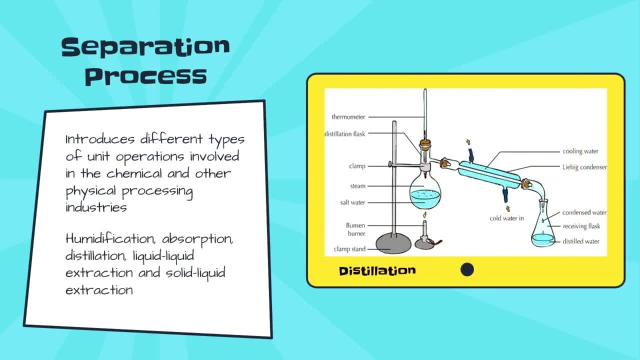 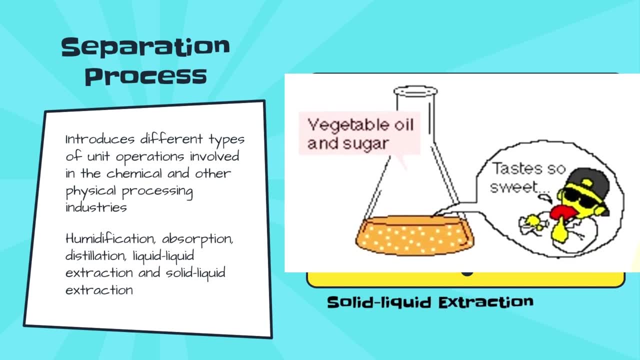 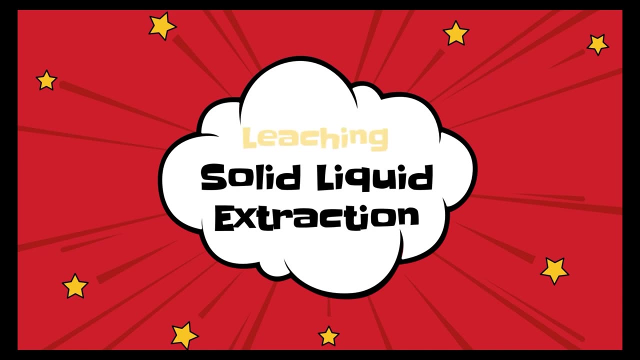 such as daddification and distillation, liquid-liquid extraction and solid-liquid extraction. Now we will discuss about the process of solid-liquid extraction. Solid-liquid extraction, also called leachate Extraction, is a crucial step in most chemical analysis. 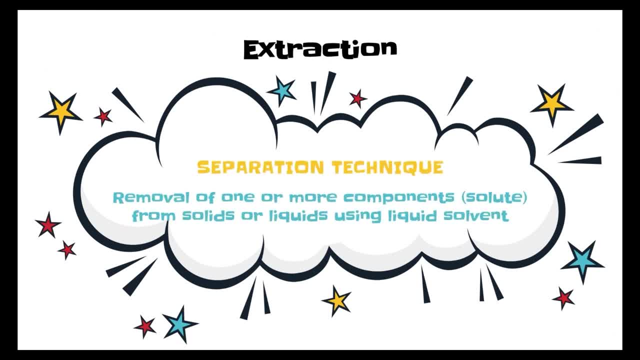 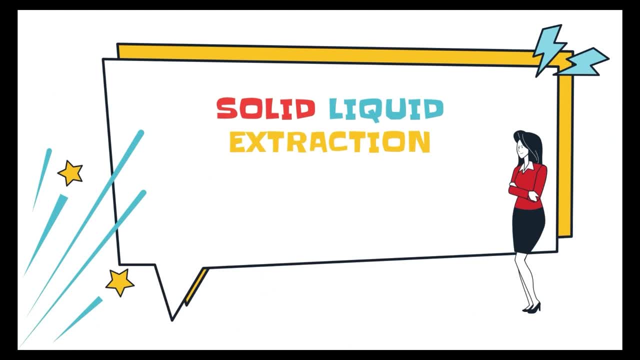 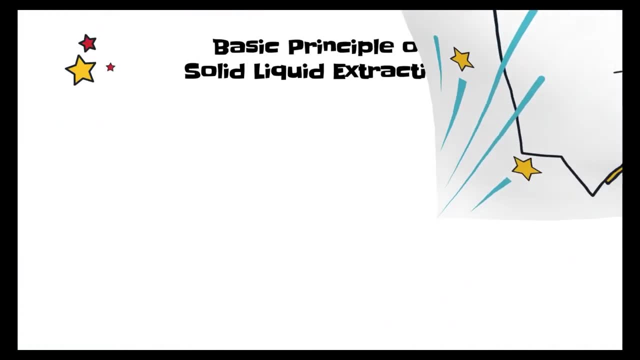 It is a separation technique which involves the removal of one or more components from solid or liquid using liquid solvent. Therefore, as the name stated, solid-liquid extraction is the separation of solid from solid by using liquid solvents. Let's look into the basic principle of solid-liquid extraction. 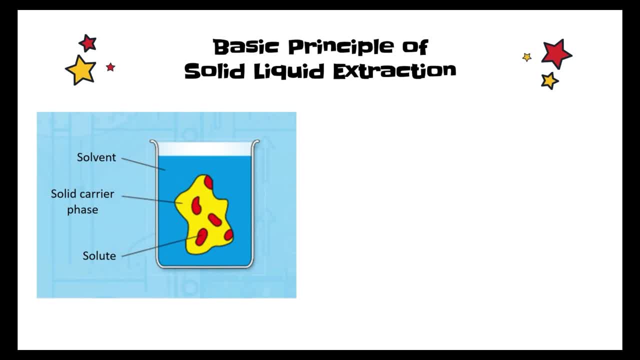 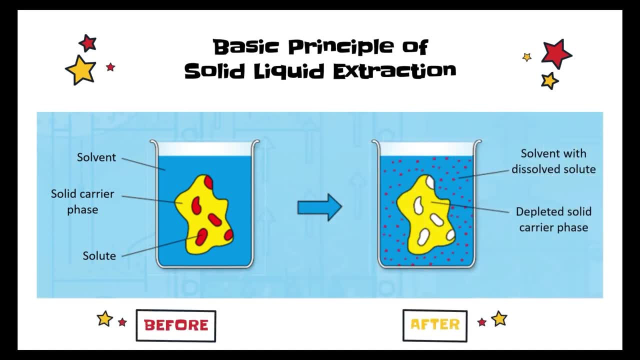 From this diagram, we can see that there is a yellow solid containing red solute immersed in the solvent. This is the condition before extraction occurs. When leaching occurs, the solute will be extracted out and dissolved in the solvent, resulting in a depleted solid carrier phase. 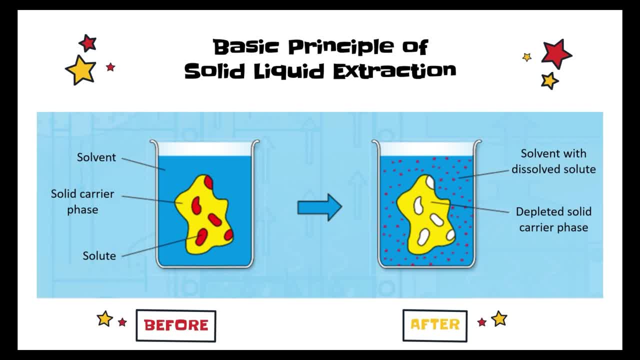 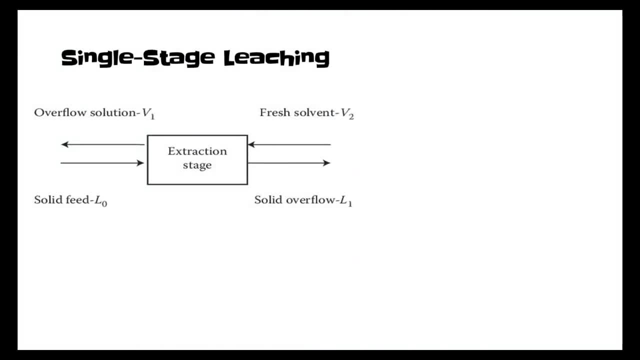 So basically, this is how the solid-liquid extraction works. Now let's look into the extraction system operations. This is a single-stage leaching process. We can see that there are two inlet and two outlet streams in this system, Where the solid feed and the fresh solvent come into contact counter-currently. 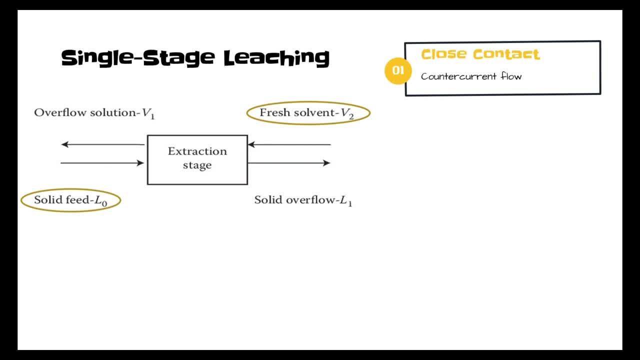 This can increase the extraction efficiency as it can increase the contact time between solvent and solute. After mixing, the solvent will extract out the solute and leaving as overflow solution, while the residual containing insoluble solid will leave as solid overflow After extracting the solute. we have to separate the solute from the solvent in order to get our product. 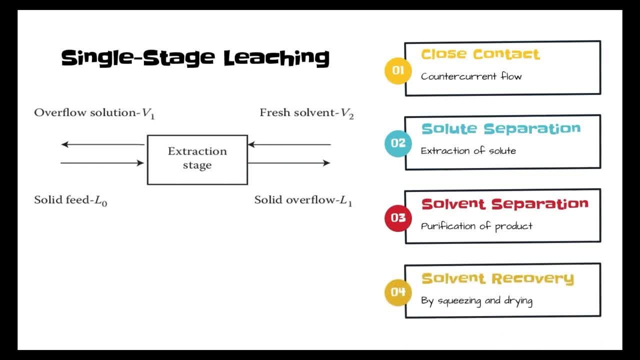 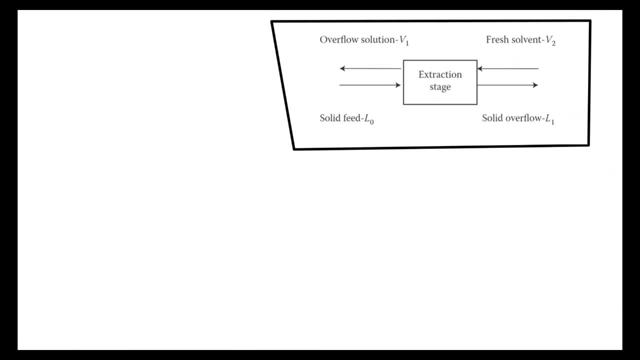 And, lastly, recovery of solvent from the moist solid by squeezing and drying to get a dry cap. This is the overall process of a leaching system and the knowledge that you may need to apply, including mass transfer and equilibrium relation. There are a few types of solvent extractor operating methods. 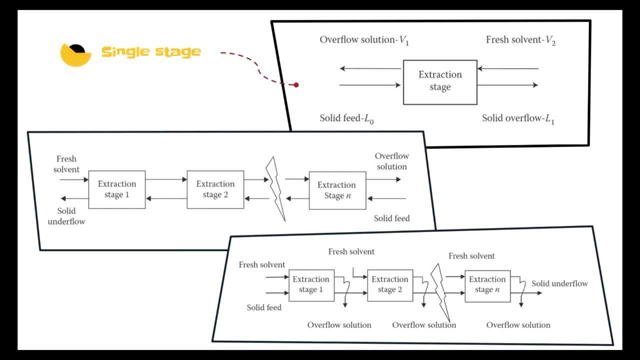 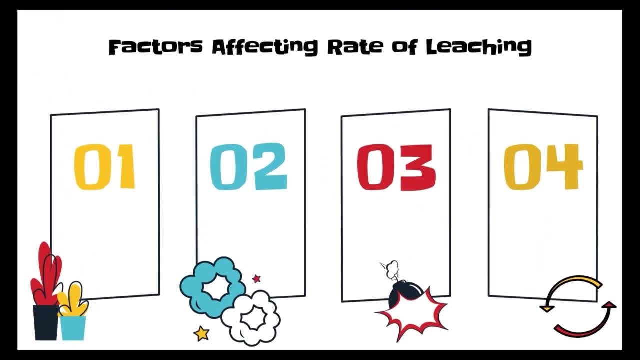 The type of flow used in leaching system can occur in single-stage or multi-stages, and it can be counter-current or cross-current. Since this is a chemical process, there must be some factors which will affect the process rate. First is the particle size. 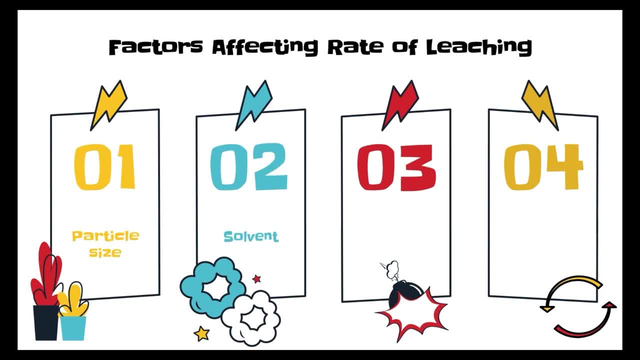 The smaller the size, the higher the transfer rate of solute. Second is the solvent. The choice of solvent must be made based on the solubility of the target analytes. Third is the temperature. High temperature can improve the extraction rate. 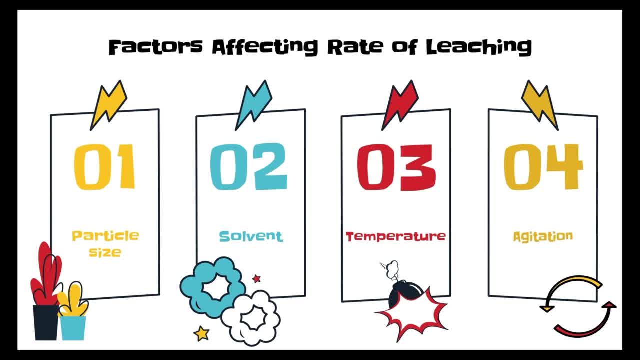 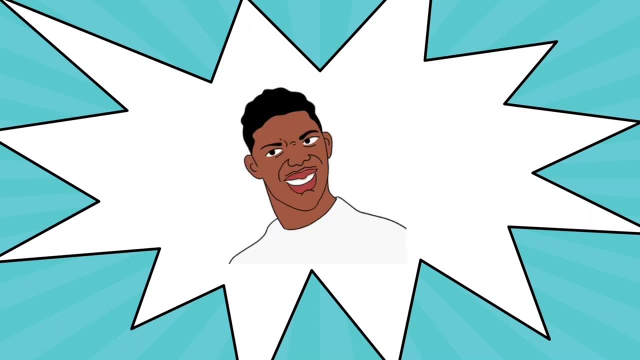 but it may cause degradation to some compound as well. Last is agitation. Agitation of the solvent will increase the turbulent diffusion and the transfer rate of material from the particle surface to the solution. Through the explanation given before, do you think that solid-liquid extraction is a complicated process? 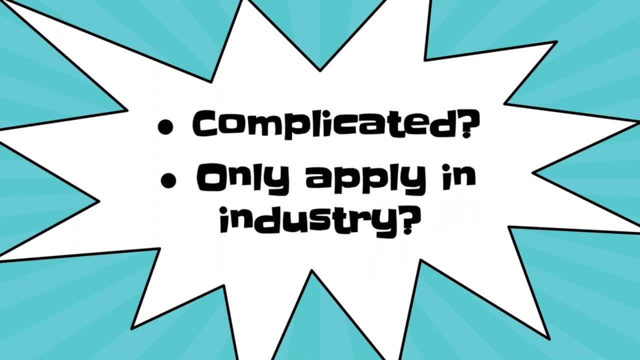 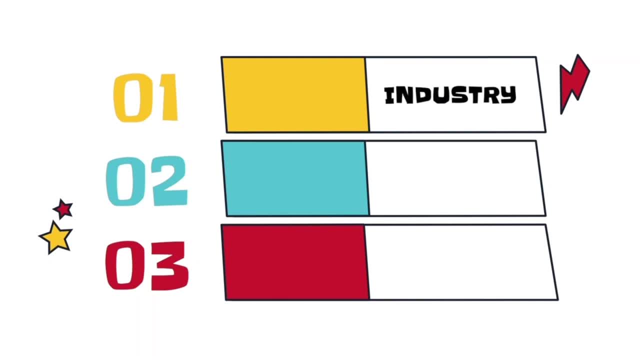 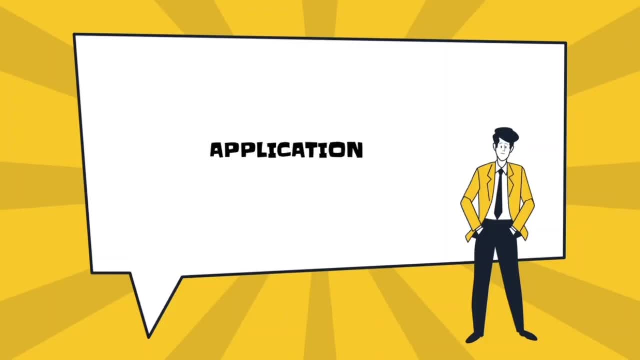 or maybe you think that it will be only applied in industry. Solid-liquid extraction is not only applied in industry, but also applied in our daily life and our environment. Now let me introduce you some applications of this chemical process. Firstly, preparation of coffee. 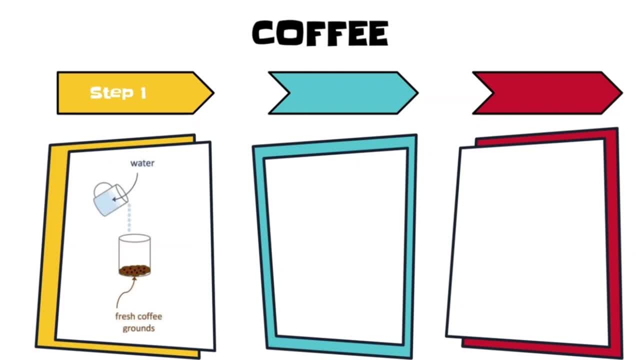 When we pour the hot water into a cup containing coffee, the water will add as solvent to separate the coffee flavors from the coffee powder. This results in drinkable coffee, which is the solvent with dissolved flavor, with the completely depleted coffee grounds remaining in the filter. 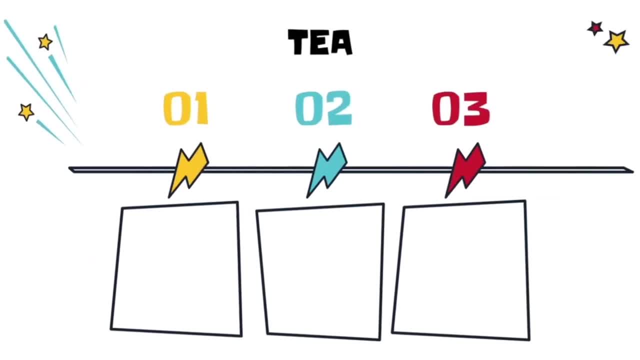 Besides, the process to prepare green tea is almost same with coffee. The green tea leaves add as solute and the hot water adds as the solvent. When the teabag meets the hot water, the hot water will extract the green tea flavors from the tea leaves. 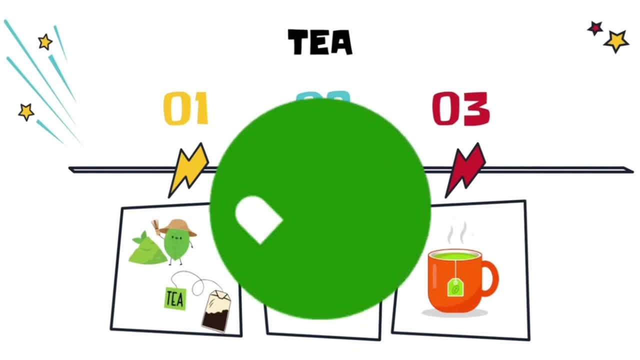 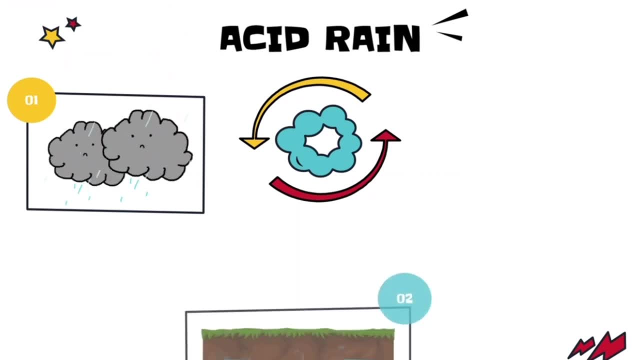 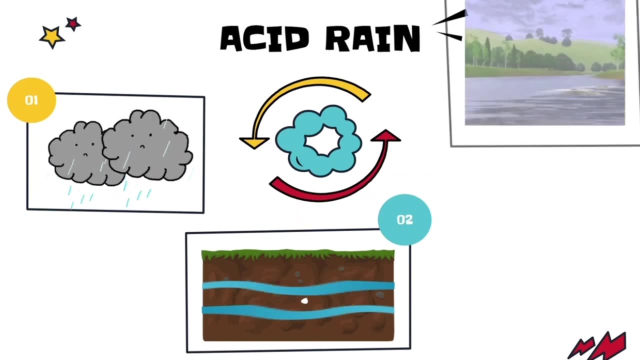 Then the preparation of green tea is done, Then acid rain is also carried out, this leaching process. As the acid rainwater flows through the soil, it adds as a solvent and will leach aluminum from soil clear particles. Then the rainwater will bring this aluminum into shrimps and legs. 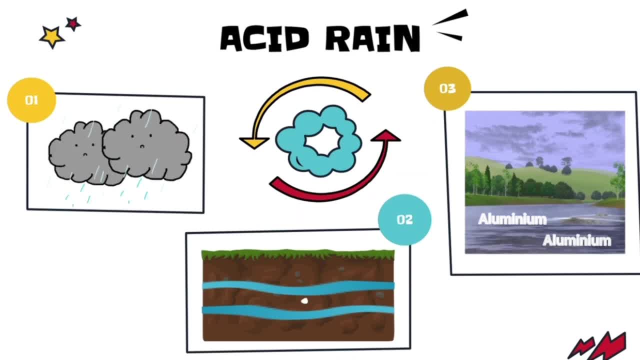 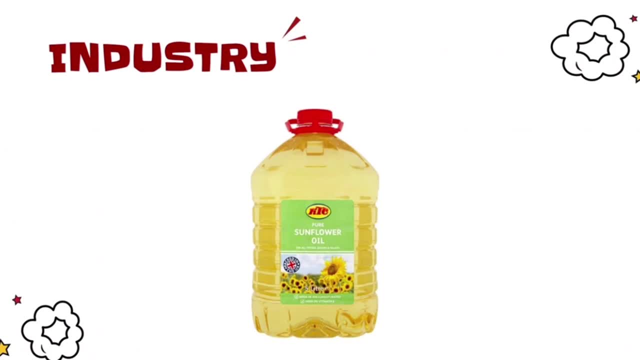 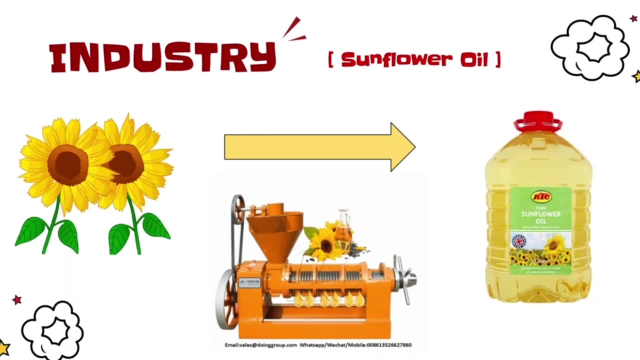 That aluminum will cause water pollution and it may be harmful to plants as well as animals. Next, are you familiar with this cooking oil? This sunflower oil is also being produced by using solid-liquid extraction. In manufacturing industry, hexane is used as solvent to extract oil from the sunflower seeds.